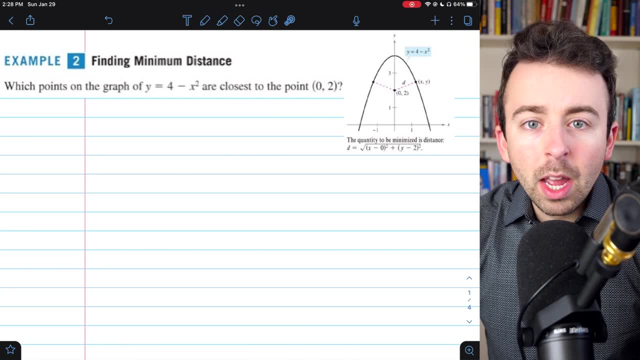 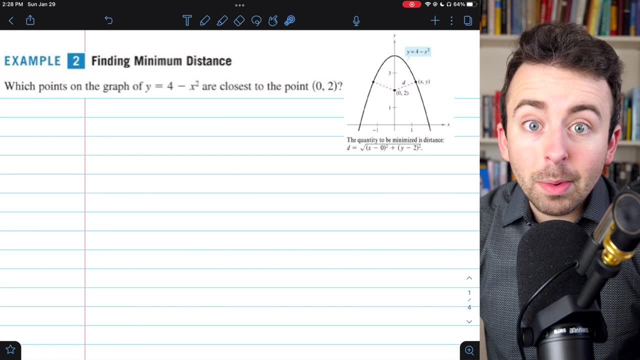 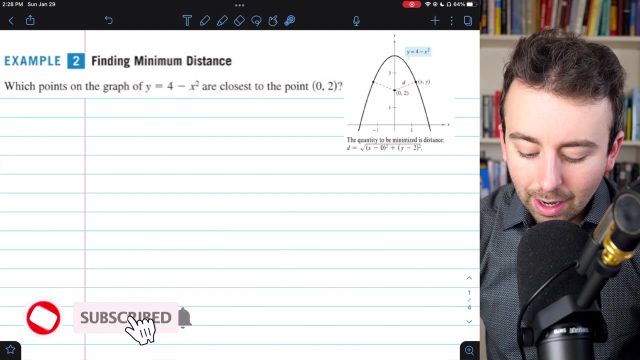 We're going to solve a common type of optimization problem where we're asked to find the points on a function that are closest to a given point. In this problem from Larson's calculus, we're asked which points on the graph of this parabola- y equals four minus x squared- are closest to the 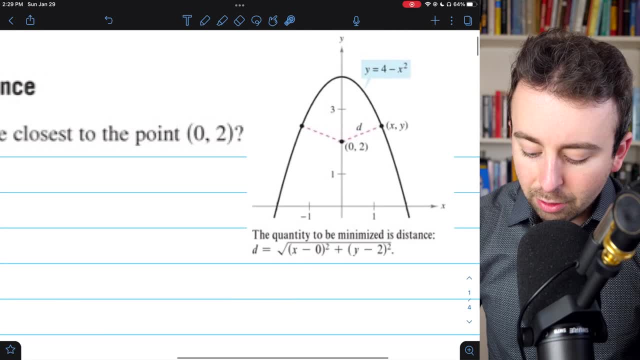 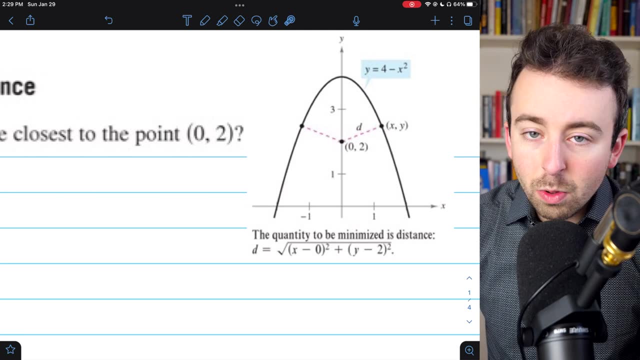 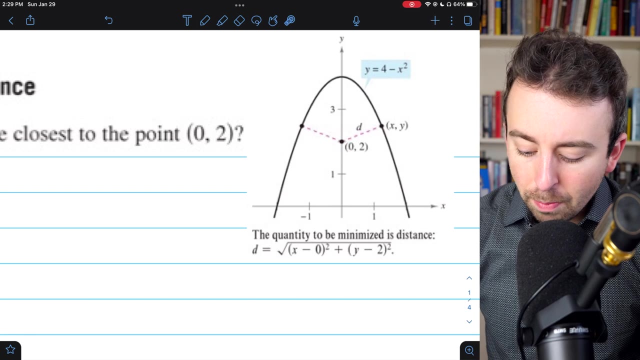 point zero two. So we can see in this figure from the textbook we've got the point zero two and we're trying to find the points on the parabola that are closest to that point zero two. So the optimizing that we're doing is minimizing the distance from a point on the parabola to the 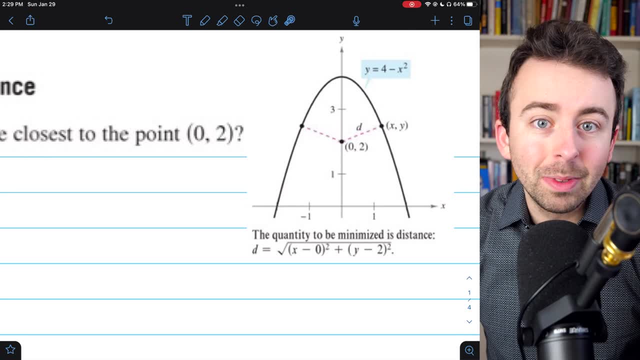 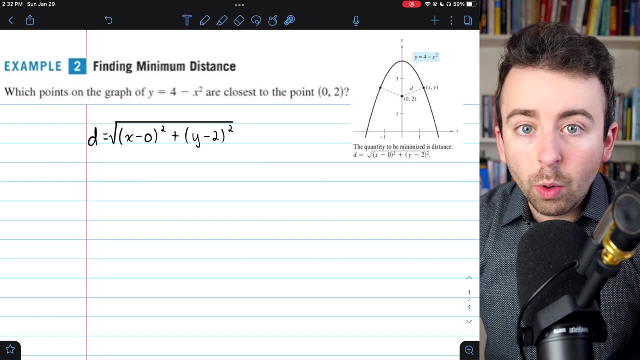 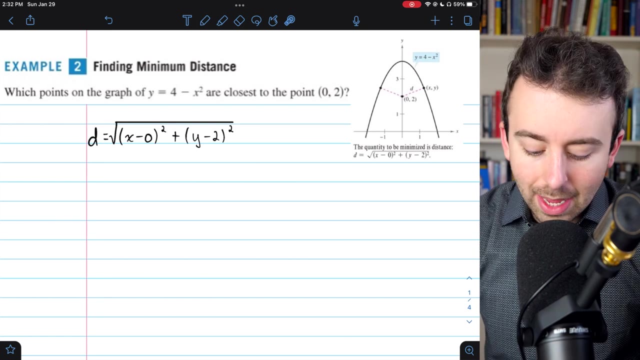 point zero two. Where do these points take on a minimum distance? To begin an optimization problem, we want to write our primary equation, which is an equation for the quantity we're trying to optimize. Again, in this case we're trying to minimize distance. So we begin with the distance formula. What we're finding the distance between is the distance. 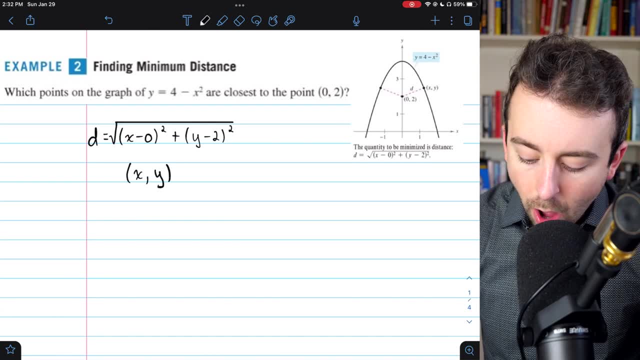 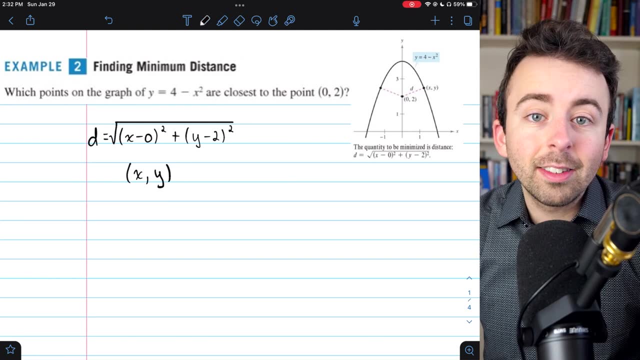 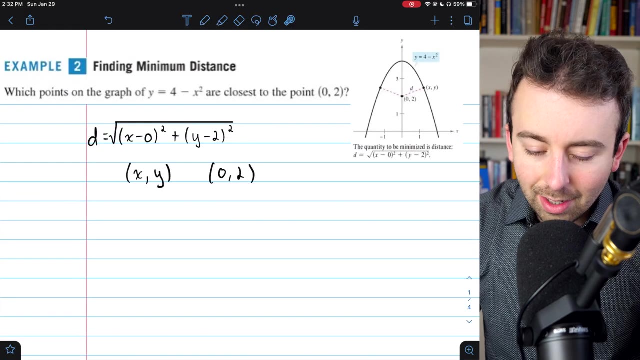 between an arbitrary point on our parabola. So this is just an arbitrary point on this curve and we're trying to represent the distance between this arbitrary point and the point in question: zero two. So this equation is the distance between those points, x and y. that comes from the arbitrary. 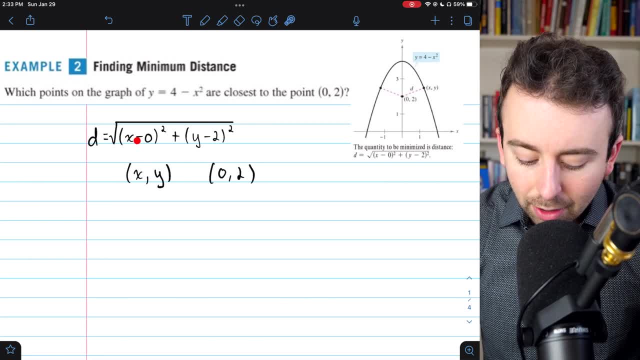 points x and y in the plane. We're trying to burnt of that data with our quadratic formula and to estimate just the distance from a point zero to 0. So it'll show up on this simulation. Then we're on our parabola And of course it's x minus 0.. 0 is the x-coordinate of the point 0,, 2.. y minus 2,. 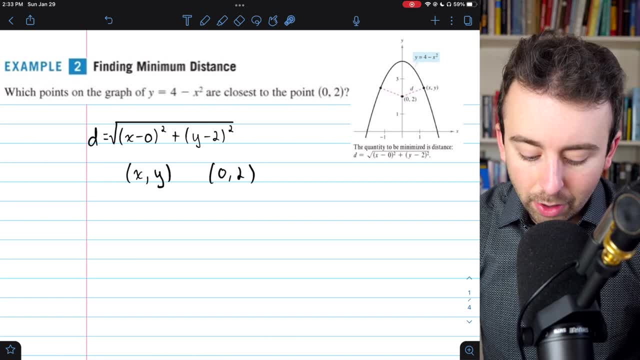 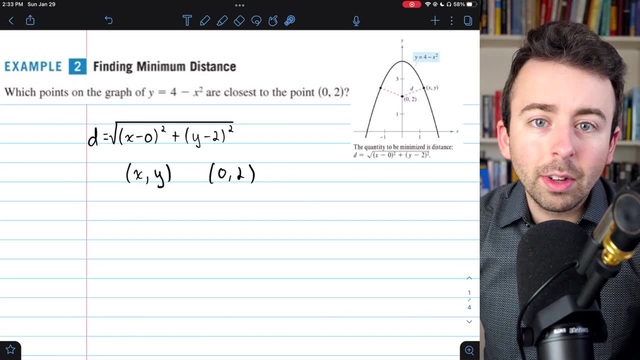 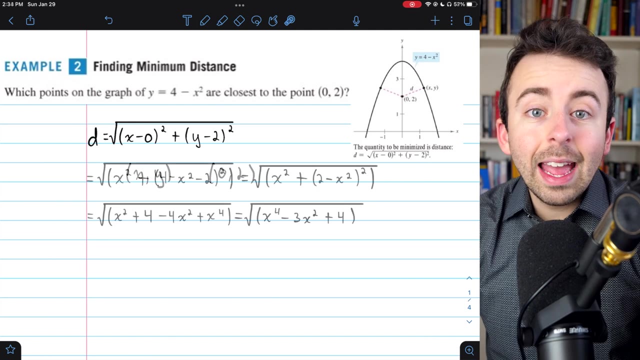 2 is the y-coordinate of the point 0, 2.. We square these differences, add them together, take a square root. This is the distance. The optimization process will have us find the x-coordinate and the y-coordinate which will minimize this quantity. And from here we just have a little. 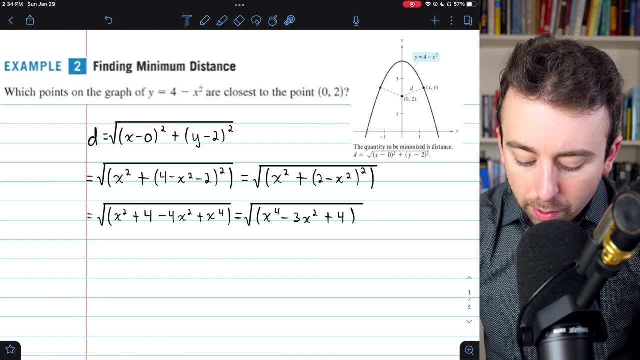 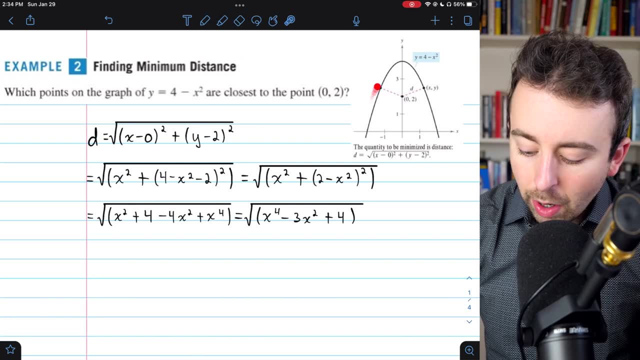 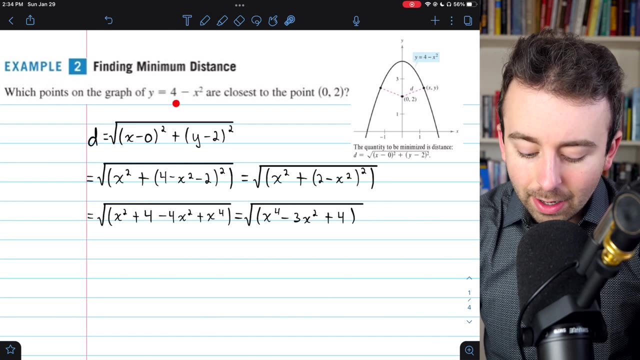 bit of algebra to do. x minus 0 squared, of course, is just x squared With y minus 2 squared. since x, y is a point on our parabola, we know that y equals 4 minus x squared, So we can replace y. 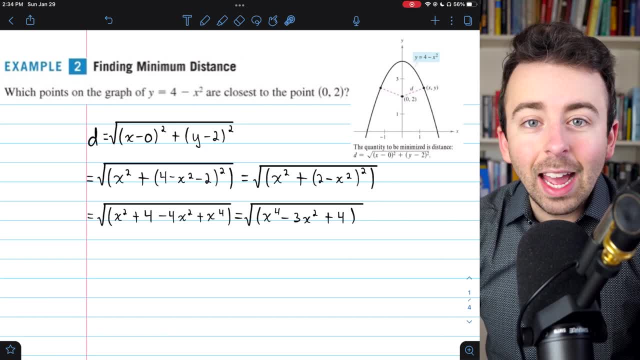 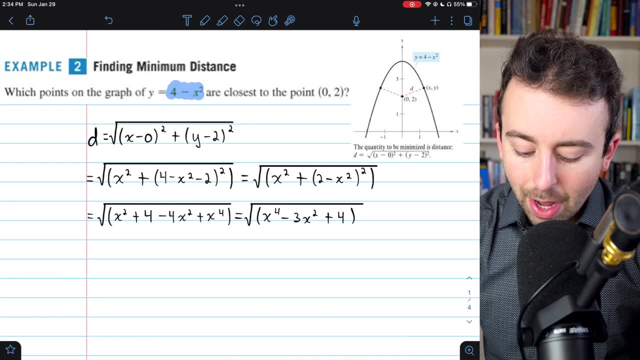 with 4 minus x squared. Again, that's because x, y is a point on the parabola, So it must be the that y equals 4 minus x squared x squared. So y minus 2 becomes 4 minus x squared minus 2.. And again this quantity is also being 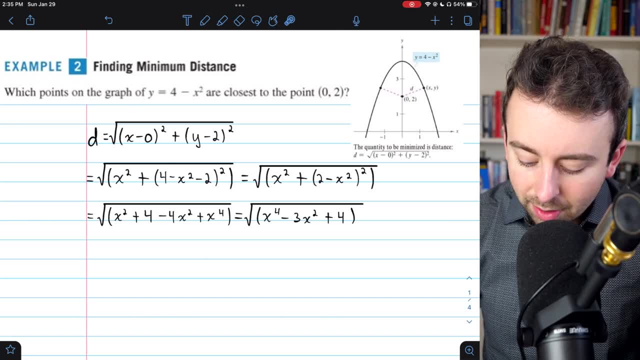 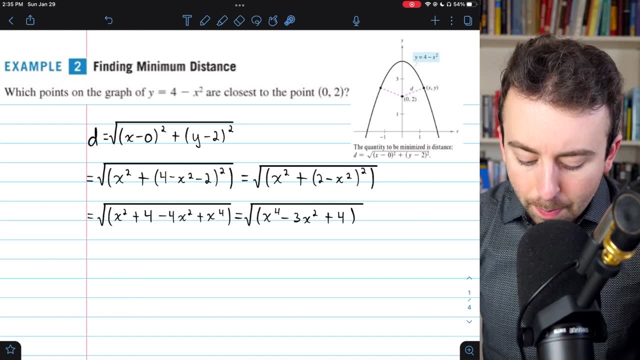 squared, Then 4 minus 2 simplifies to just 2.. And at this point we can expand 2 minus x squared. squared, That becomes 4 minus 4x, squared plus x to the fourth. And then simplifying again by 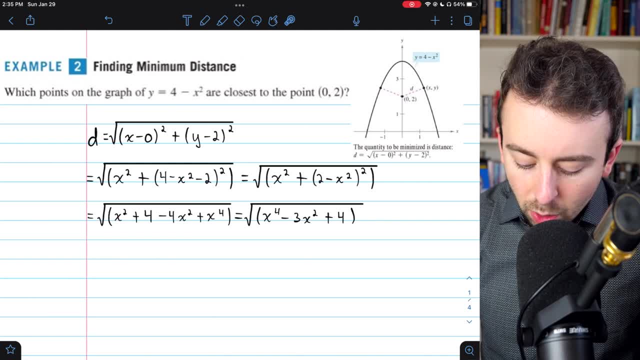 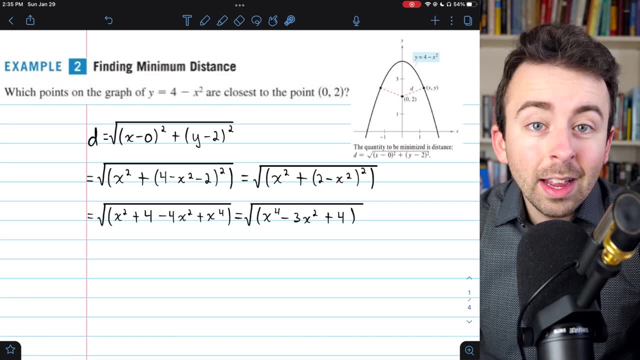 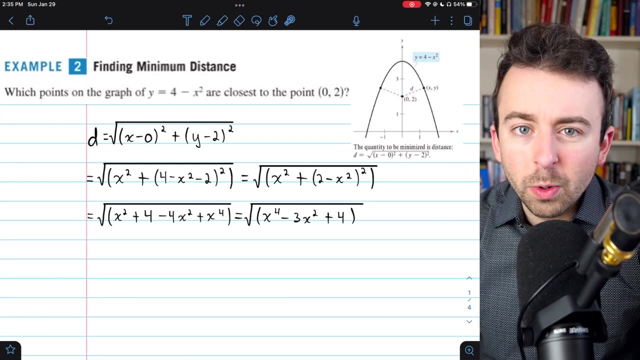 combining x squared and minus 4x squared, we get x to the fourth, minus 3x squared plus 4.. This, of course, is all in a square root. Now, remember, we're trying to minimize this distance, So in fact, we don't really have to worry about the square root, because where the square root of 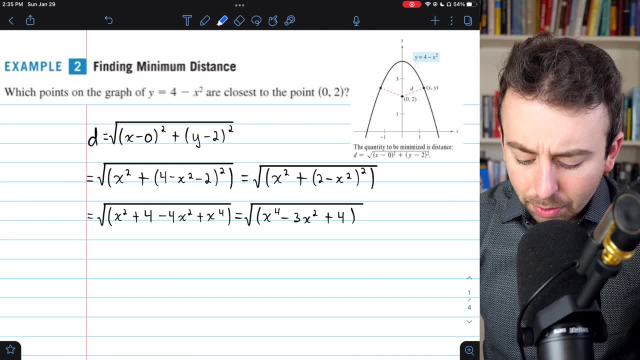 this expression will be minimized is simply wherever this expression in the square root will be minimized. So we can just focus on the thing that's important to us And that's the square root of the square root. So we can just focus on the thing that's important to us And that's the square root of the square root. 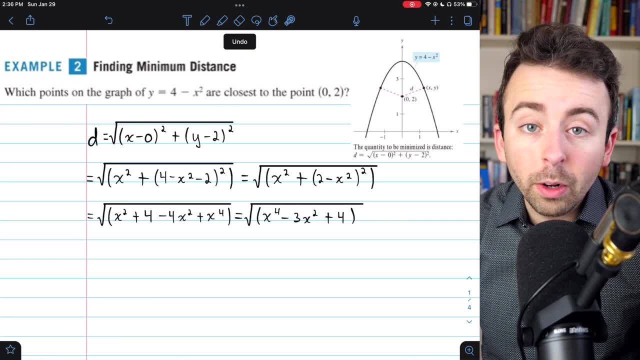 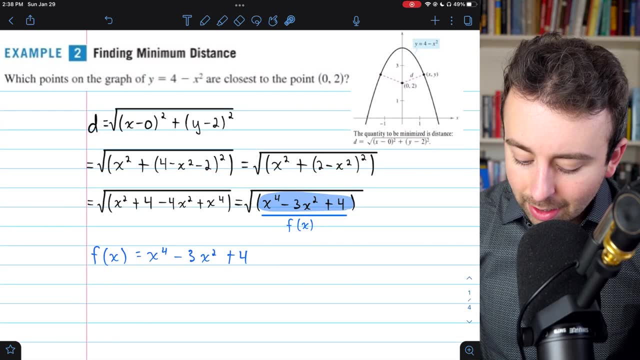 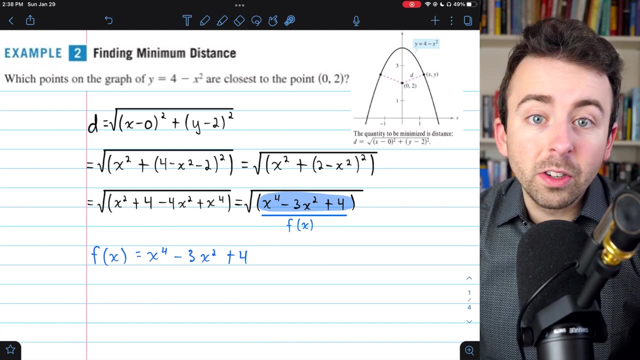 If we can minimize that, that will, of course, also be where the square root takes on its minimum value. So this expression under the radical is our f of x, And we're going to try to minimize this. It's important that we take a second to consider our domain, though, In an optimization. 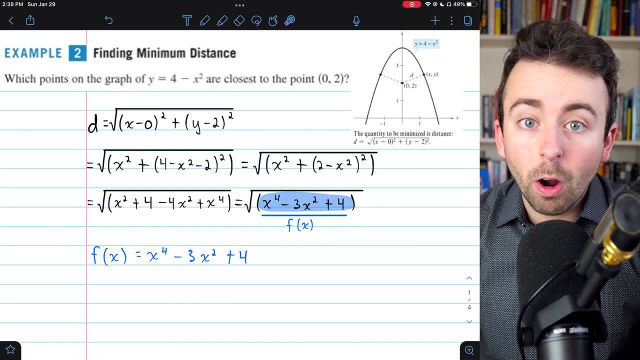 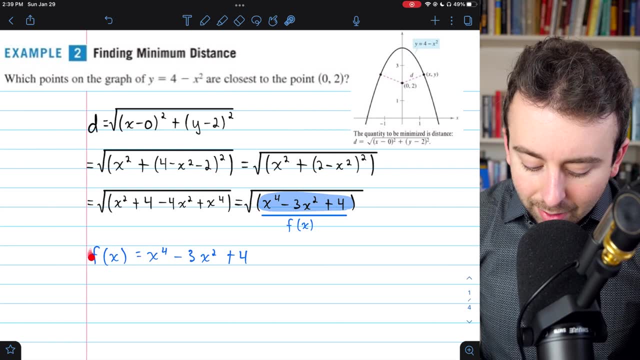 problem. you need to check the endpoints of the domain, if there are any. In this case, our domain is all real numbers, So there are no endpoints to check. Of course, f of x is just a polynomial, So its domain is all real numbers And there are no contextual restrictions. 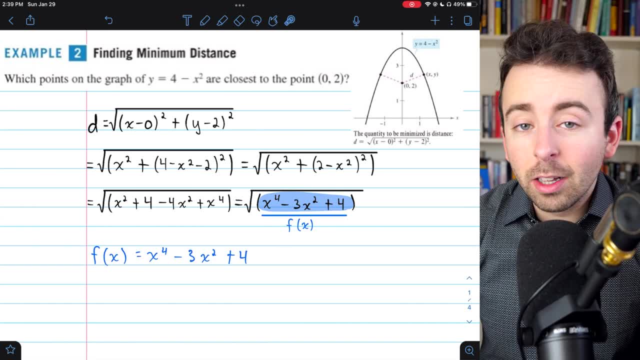 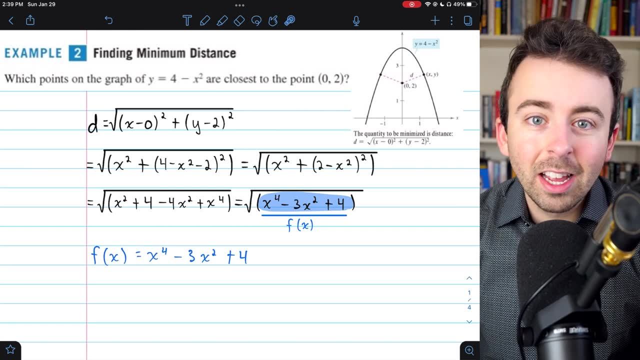 in this problem that we would have to place on the domain. In a lot of problems you might not want x to be negative, for example if x is representing the side of a box, But in this case there are no such restrictions. Even with the distance equation, x could be anything. And since 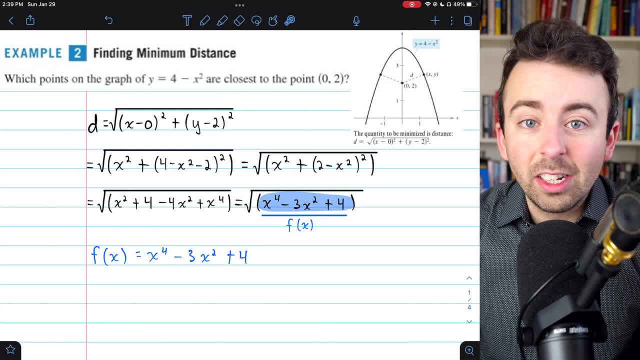 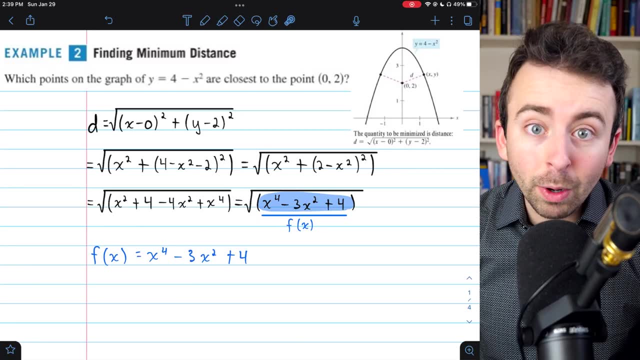 we have these quantities being squared, the distance would still be defined, So the domain is all real numbers. We don't have any real numbers. We don't have any real numbers, So we don't have any endpoints to check. We can proceed with finding the critical points of this function. 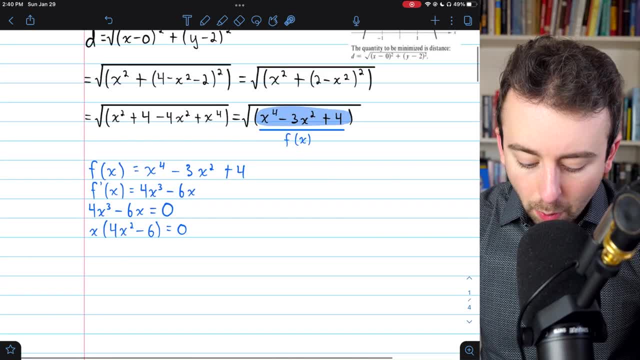 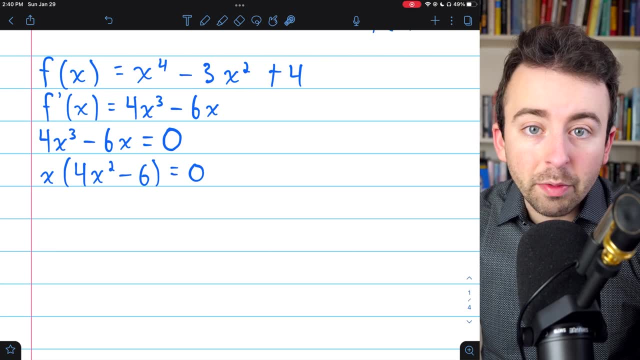 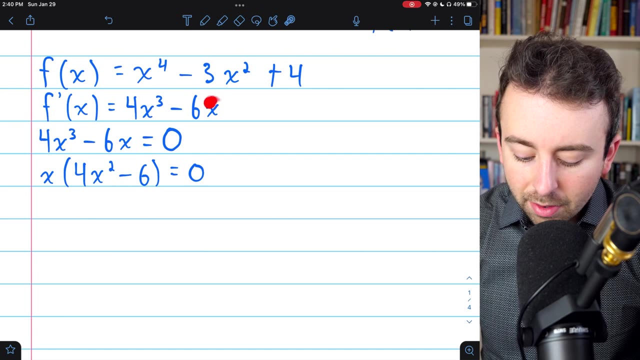 in order to find its minimum values. So we're now just going through the usual process for finding extreme values of a function: We take our function and then find its derivative. This is just a couple applications of the power rule. x to the fourth becomes 4x cubed. 3x squared becomes: 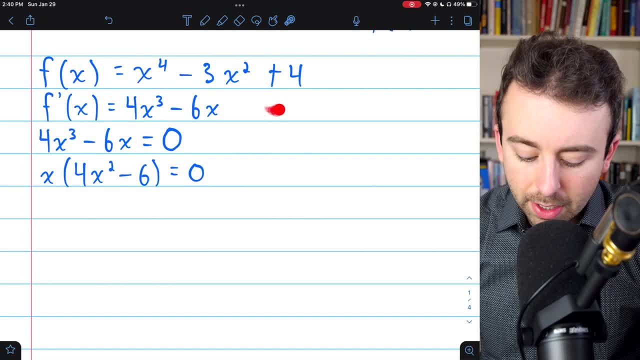 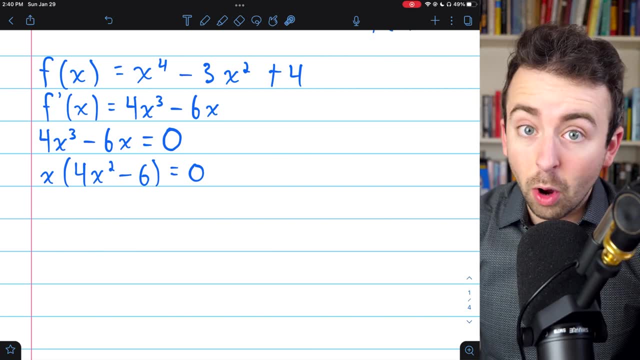 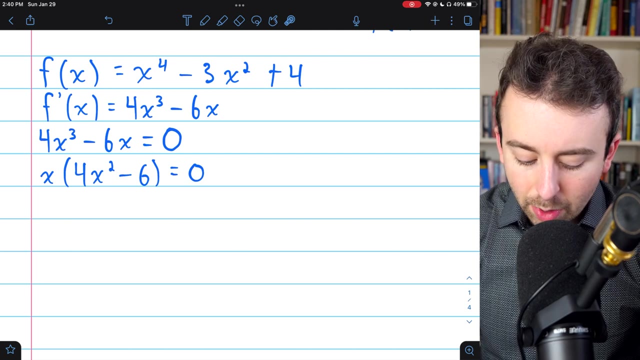 6x, And of course we are subtracting Plus 4 just becomes 0.. Now to find the critical points we have to consider. where is this derivative? undefined, Nowhere. Okay. so then set it equal to 0 and let's solve for x. To do that, just factor out an x, So we have x times 4x squared. 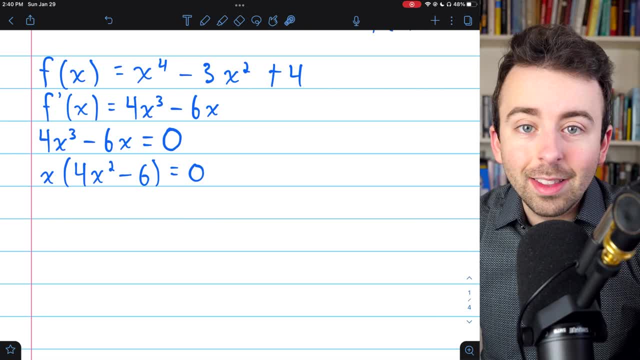 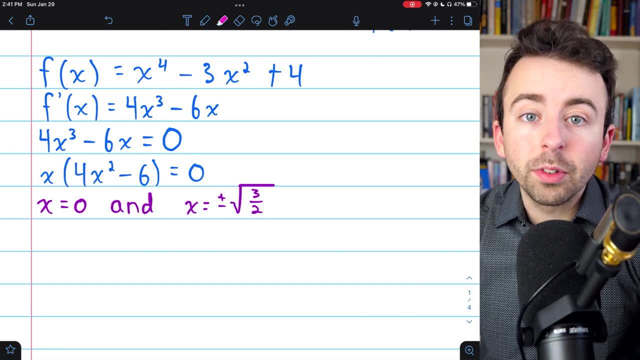 minus 6 equals 0. And then apply the 0 product property. In order for this product to equal 0,, it must be that either of the factors are 0. If we set this factor equal to 0, then of course, 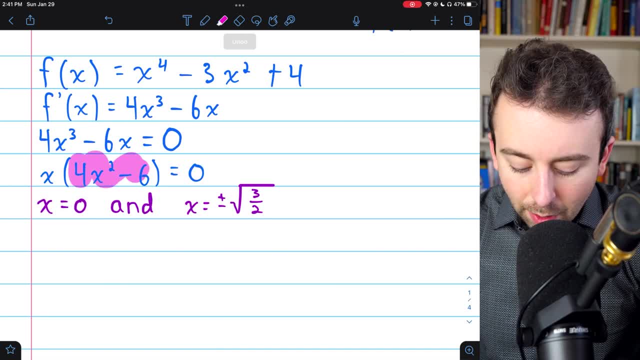 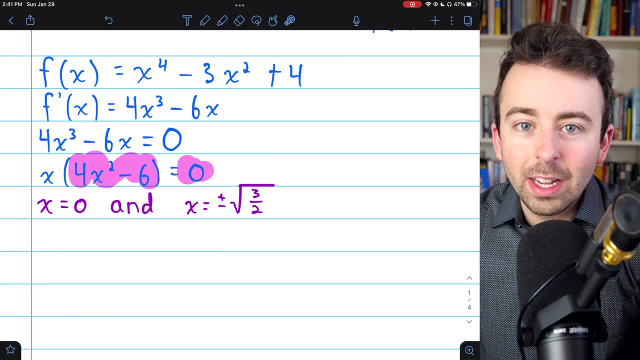 we get that x equals 0.. If we set this factor equal to 0, then we would add 6 to both sides, divide everything by 4.. So x squared equals 6 fourths, or 3 halves, And then just take square roots And so we get that x. 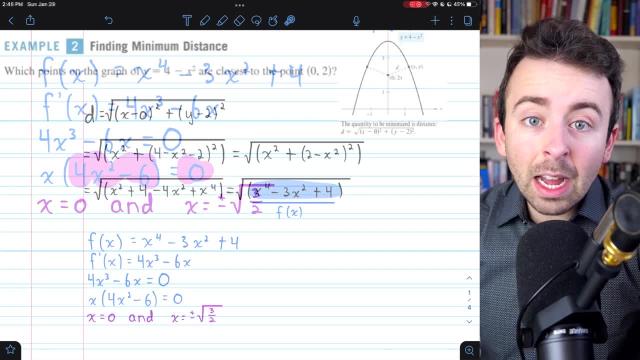 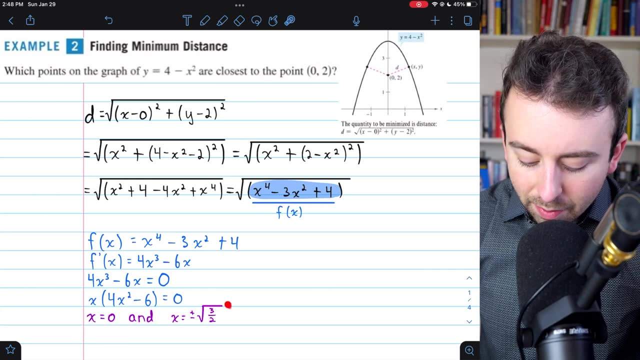 equals plus or minus the square root of 3 halves. Now that we found the critical points of our function, all that remains is to use the first derivative test or the second derivative test to classify these as mins, maxes or 0s. 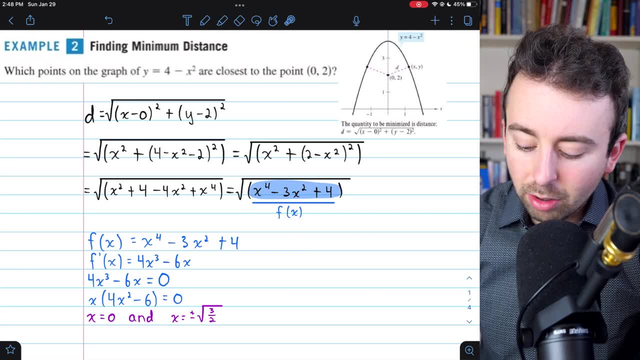 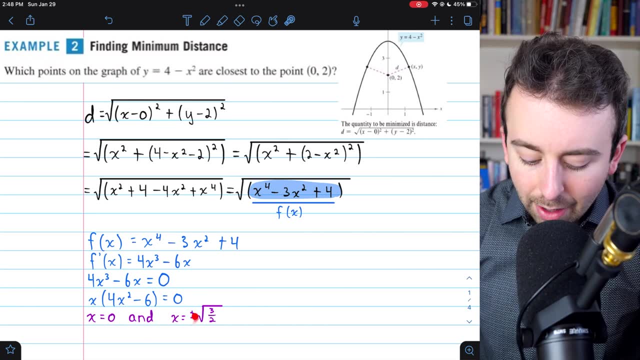 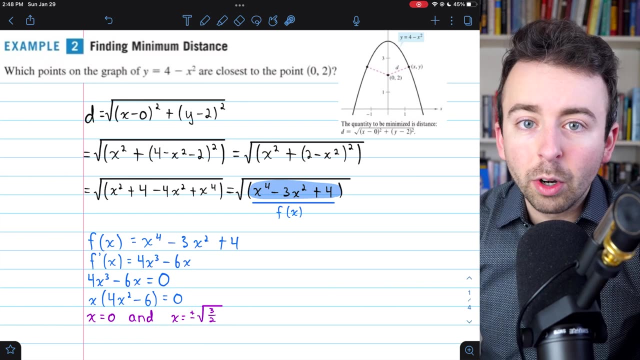 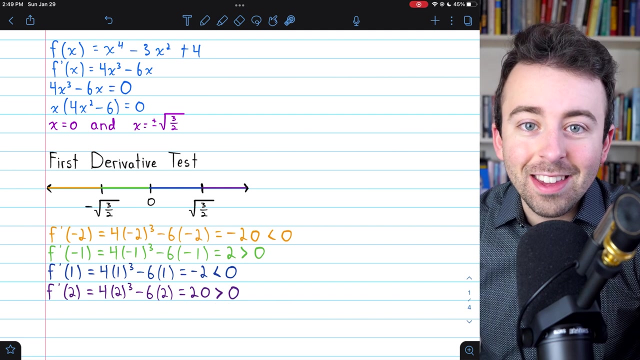 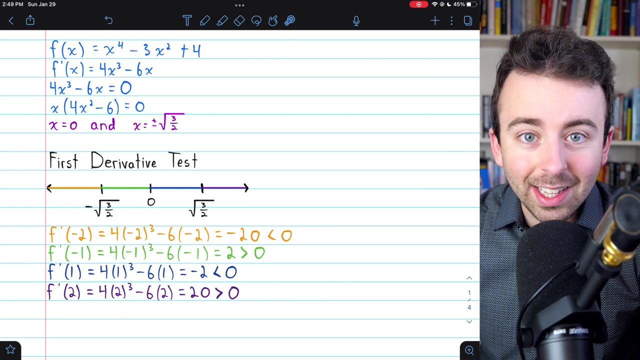 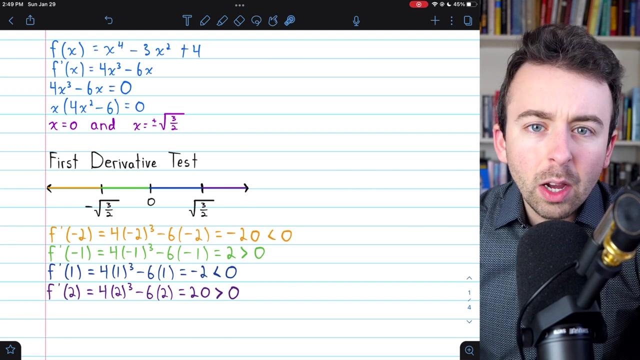 And here's my color-coded application of the derivative test. I've sketched out here a number line just to represent the intervals between the critical points. So the only things I've marked on here are the critical points And to use the first derivative test, we want to see what's happening to the function. 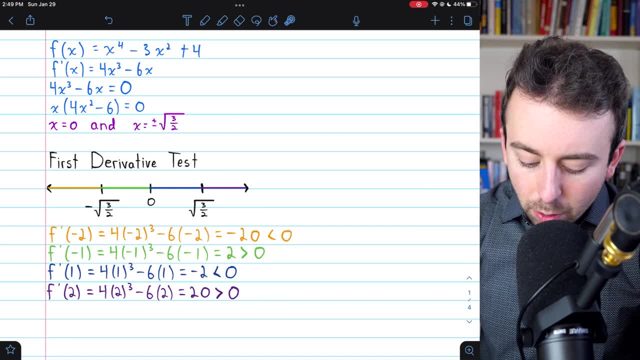 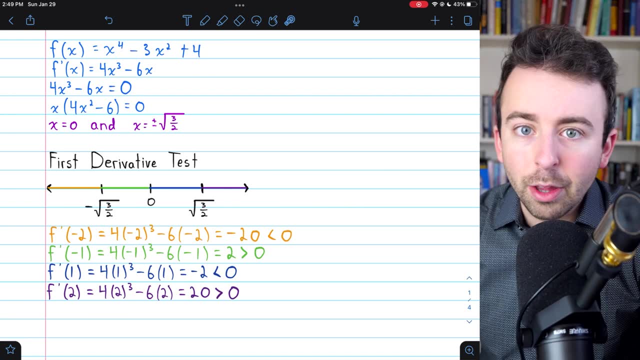 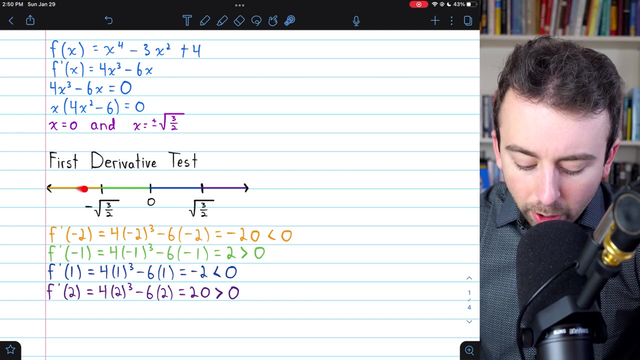 Is it increasing or decreasing on each interval between the critical points? To do that, we simply take a number from each interval and plug it into the derivative. If the derivative is positive at that point, then the interval must be increasing. For example, in this orange interval from: 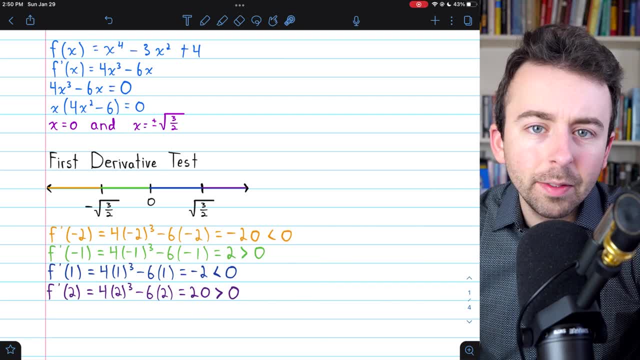 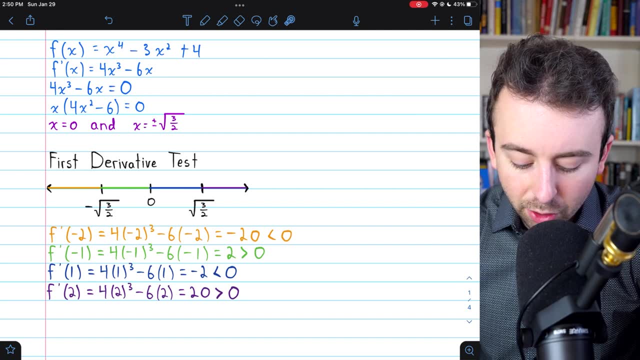 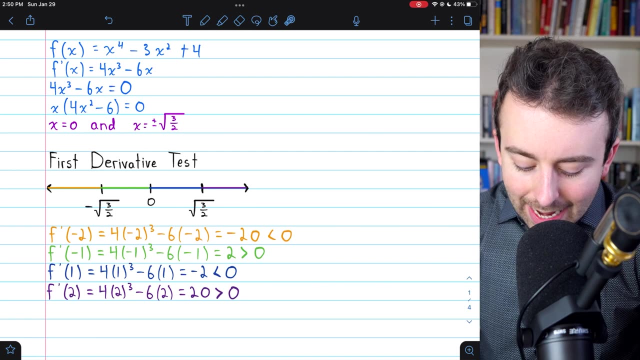 negative infinity to negative root, 3 halves. I just have to take any point from that interval. I know that negative 2 is in this interval, since negative 2 is less than negative square root of 3 halves. And if I take negative 2 and then plug it into the derivative, this is what I get: It's negative 20,. 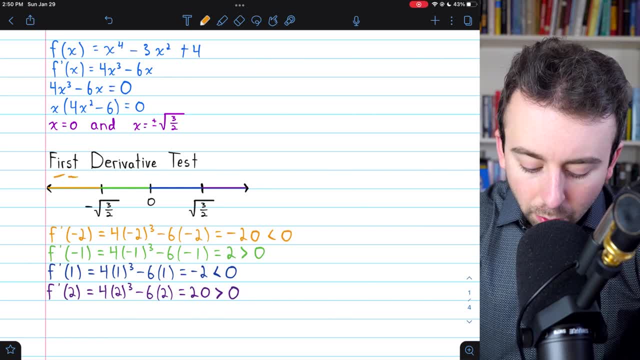 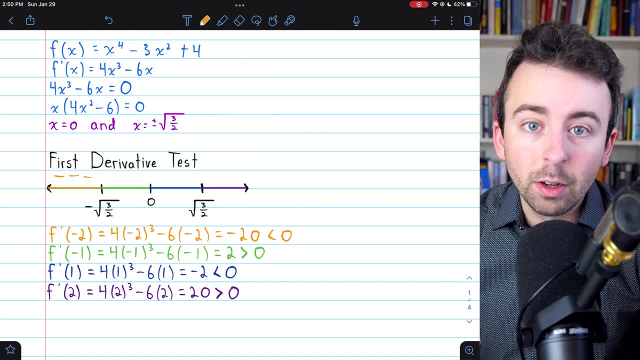 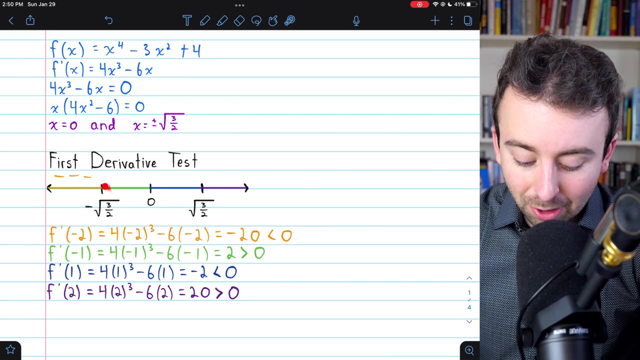 which is less than 0. That means on this whole interval the function must be decreasing. It can't switch from decreasing to increasing on the interval because to do that it would have to cross through 0. But we know the derivative doesn't cross through 0 until the critical point. 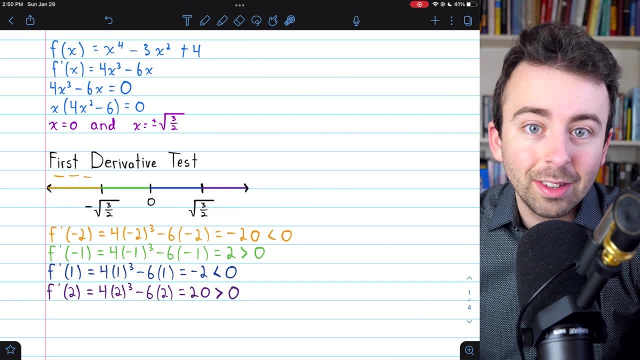 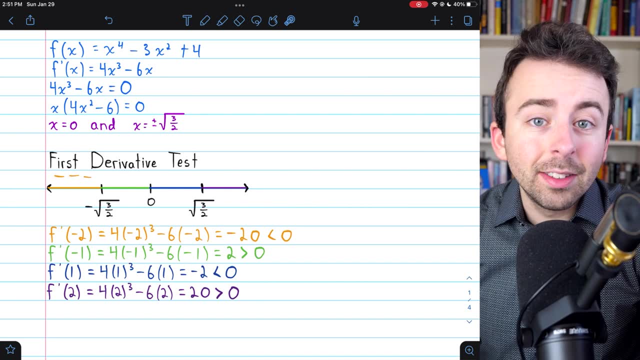 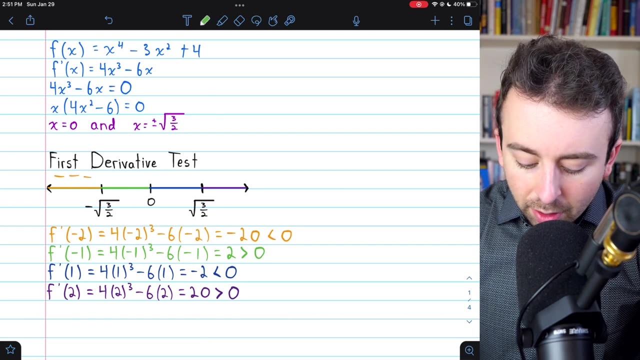 So this whole interval must have the function decreasing. Then we take a point between negative root 3 halves and 0. A point in this interval is negative, 1, for example. So we plug that into the, which is positive. So on this whole interval the derivative is positive and thus the function. 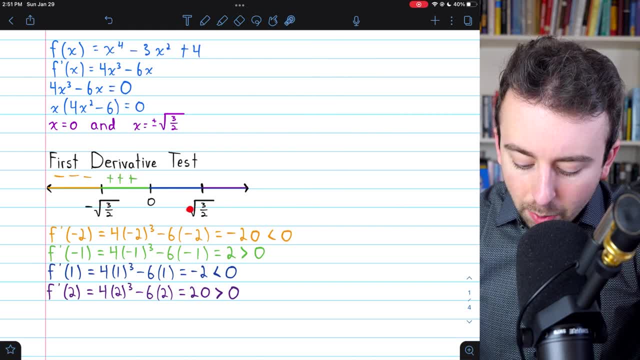 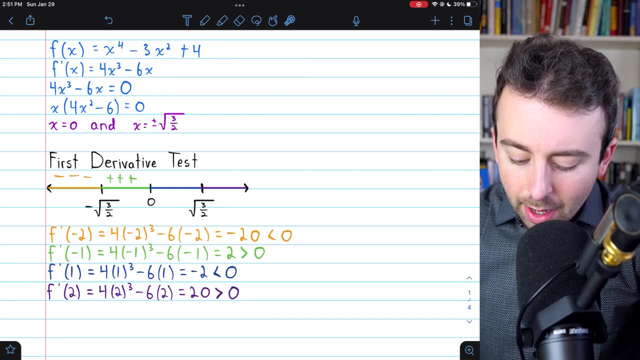 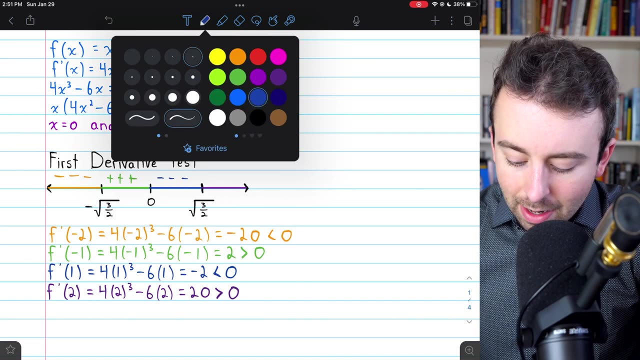 is increasing Then between zero and the square root of three halves. positive one is in that interval, So we plug in positive one and we get negative two, which is less than zero. So the function is decreasing on that interval. Similarly, on this final interval from root, three halves to, 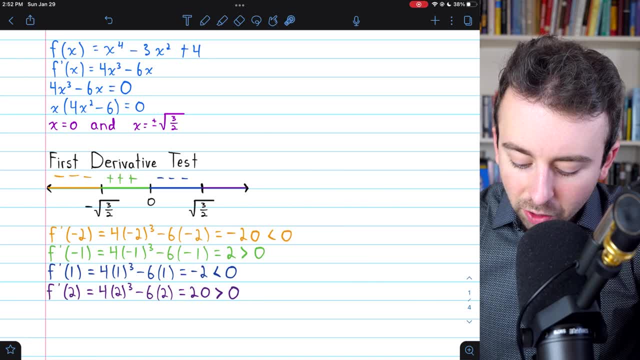 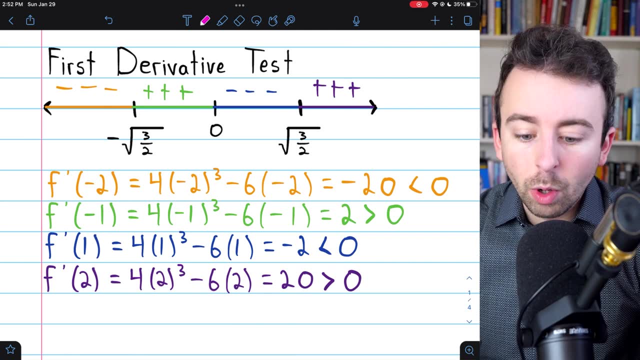 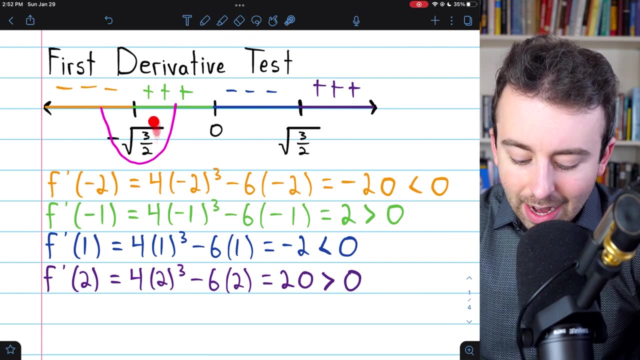 infinity. we plug in two and find that the function is increasing. Now how do we use this information to determine where the mins and maxes are? Well, what we see is the function is decreasing and then increasing. at x equals negative root. three over two. It switches from decreasing to increasing. 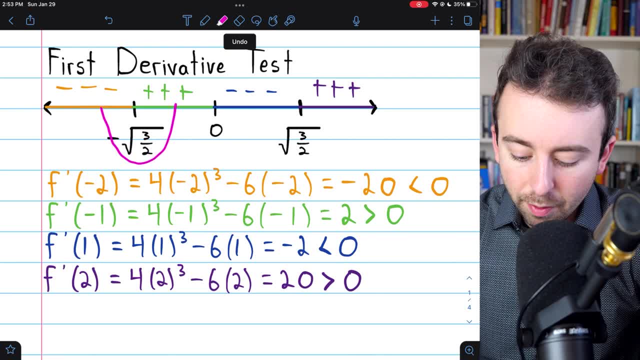 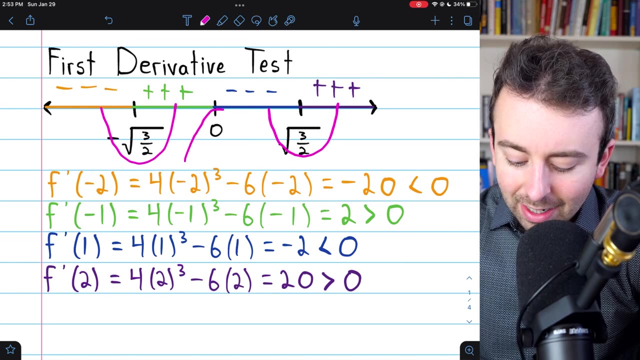 So clearly that has to be a minimum of the function. Similarly, for positive root three over two, the function is decreasing Then increasing, So we must have a minimum there. at positive root three over two, On the other hand, at x equals zero, the function is increasing then decreasing. So there we would have a maximum. 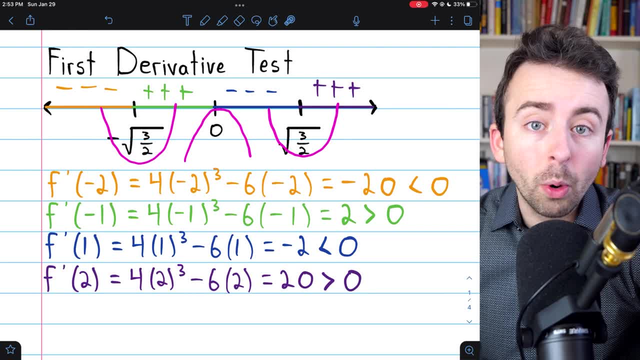 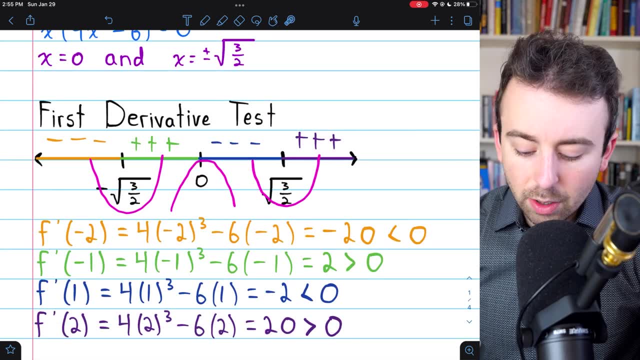 Now, remember, we're trying to minimize the distance, So the two points we're actually interested in then are positive and negative root three over two. So we know that x equals plus or minus. root three over two are minimums, But it could be that one x gives us a point. that's 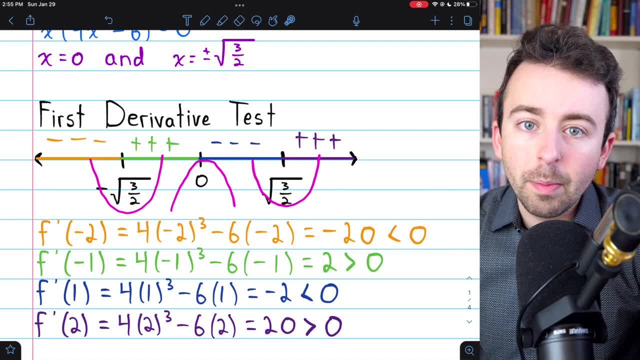 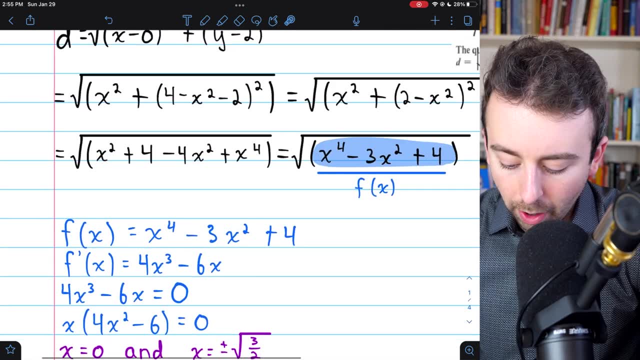 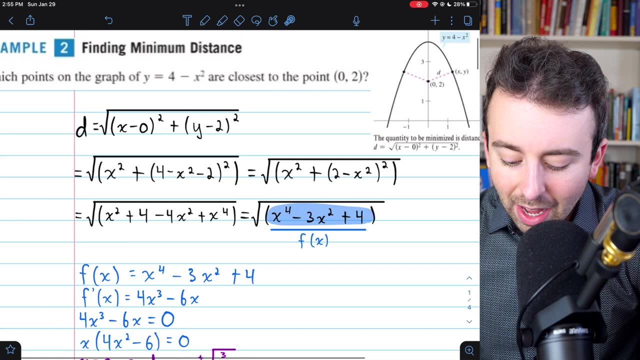 actually closer to zero two than the other, even though they might both be minimums. So we would have to plug these into the distance formula that we had before to see which one actually gives the smallest distance. However, in this case, we can notice that what we've got here is an even. 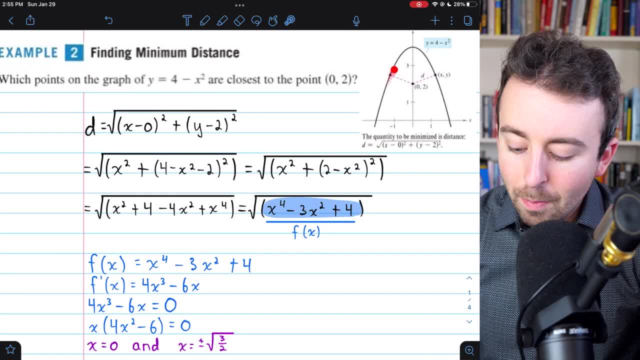 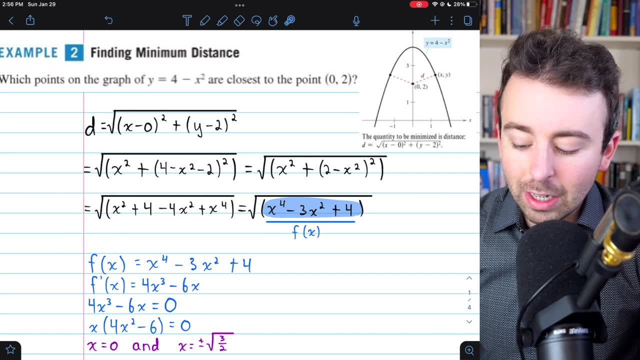 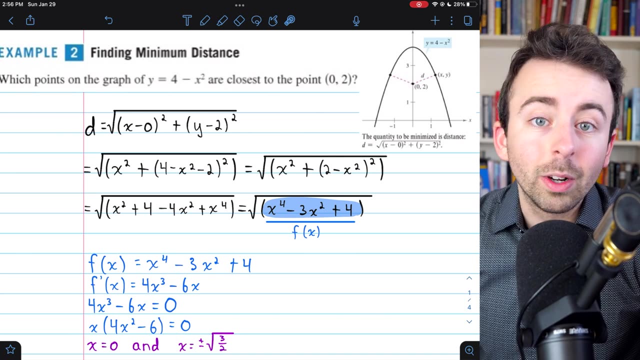 function. This parabola is symmetric about the y-axis. It's symmetric about x equals zero. So we know that the distance from zero two is going to be the same for positive root three over two as it is for negative root three over two, because this is an even function, symmetric about the y-axis. 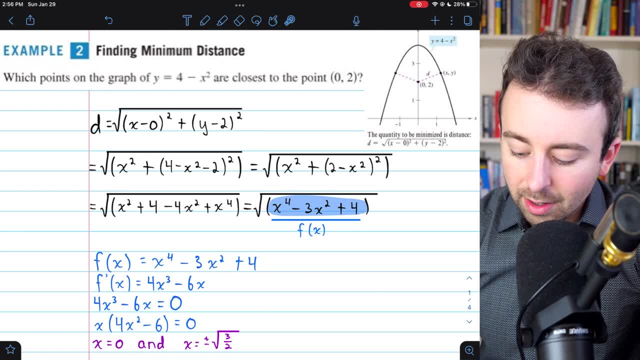 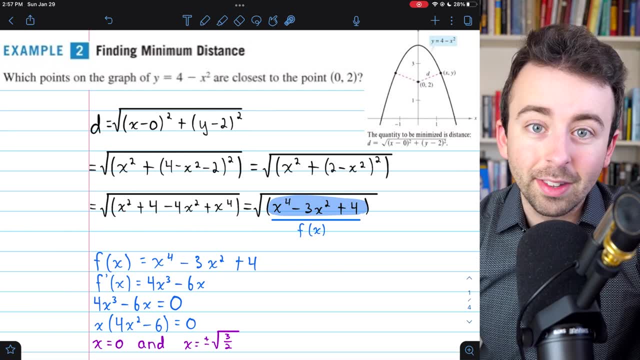 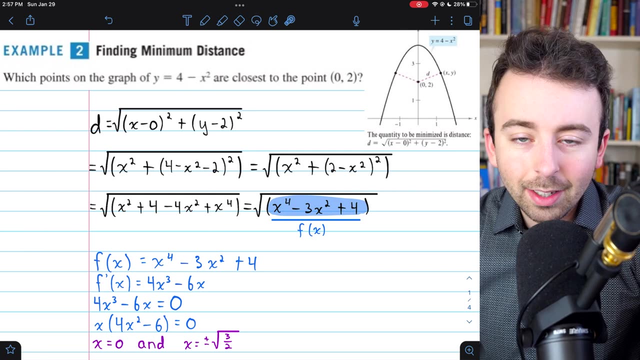 Since the symmetry of the parabola guarantees us that the distance from zero two to the point where x is positive and negative root three over two will be the same. those will be the same minimum distances. All that remains is to take those x values and plug them into the parabola to 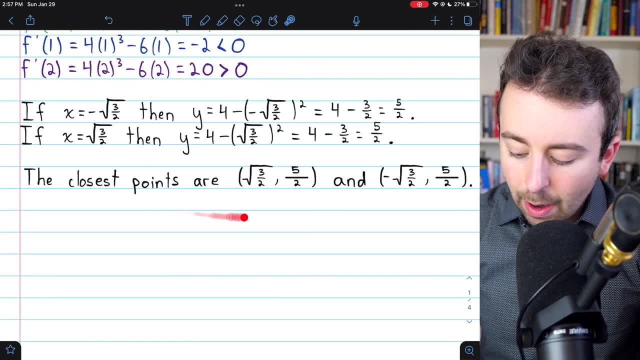 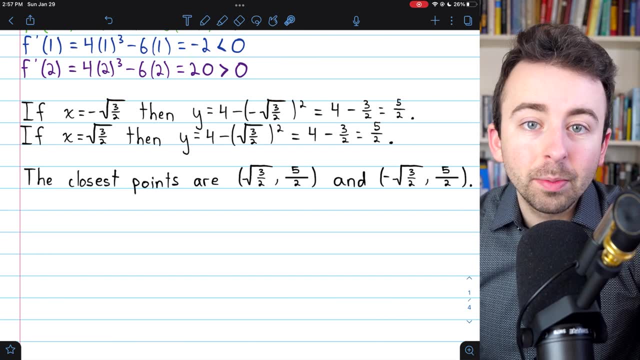 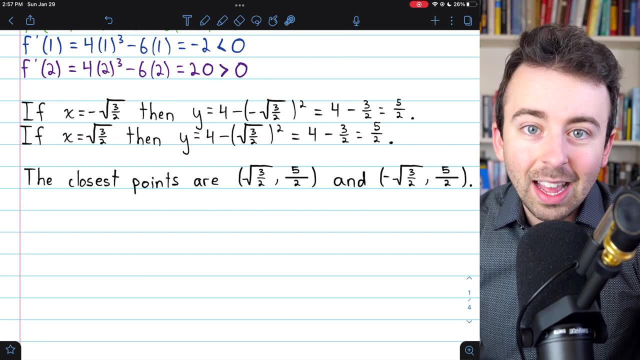 see what the y-coordinate is, And doing that, here is our conclusion. For x equals negative root three over two. the y-coordinate on the parabola is five halves And of course, since it is symmetric, the y-coordinate is five halves for positive root three over two as well, And so 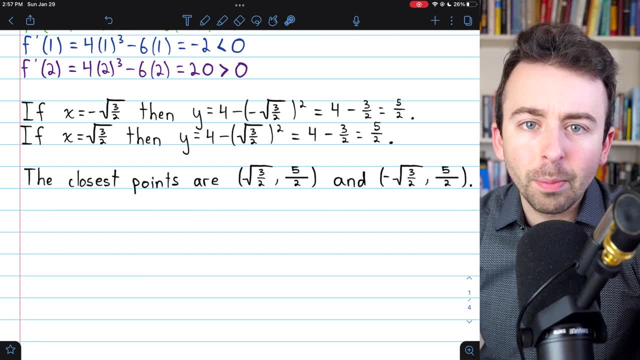 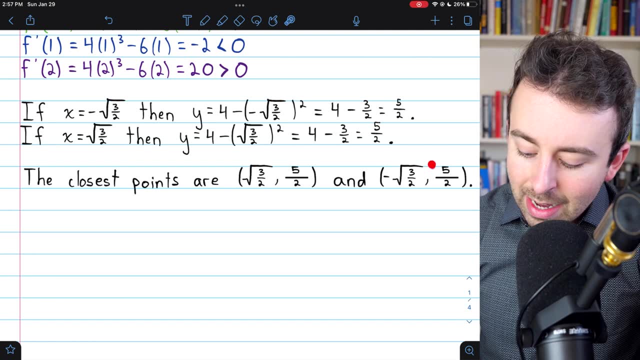 these are the two points on the parabola closest to the point zero two, which was the original question. The closest points are root- three halves- five halves and negative root- three halves- five halves. Hope this was helpful. Let me know in the comments if you have any questions.